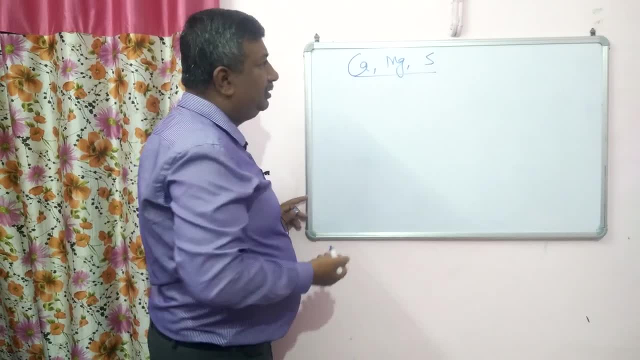 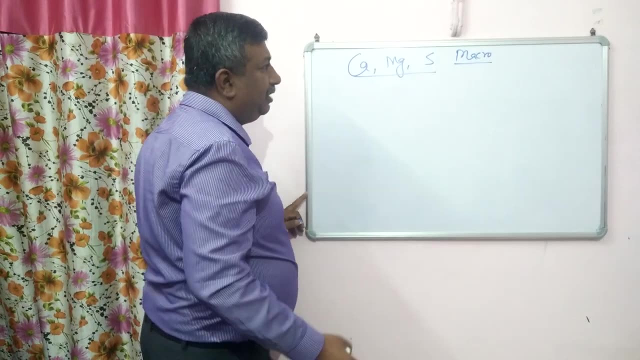 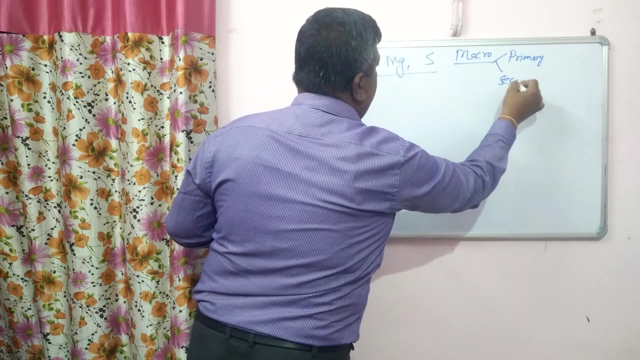 and these are secondary nutrient. these are micronutrient. micronutrients are CHO, NPK and calcium, magnesium and sulphur, and macro are divided into two groups: primary nutrient and secondary nutrient. Primary nutrient are N, P and K, while secondary nutrient are 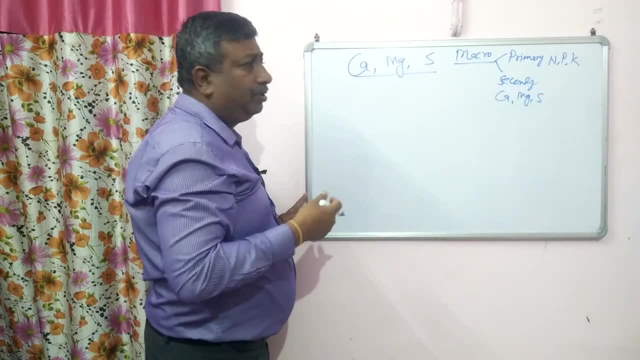 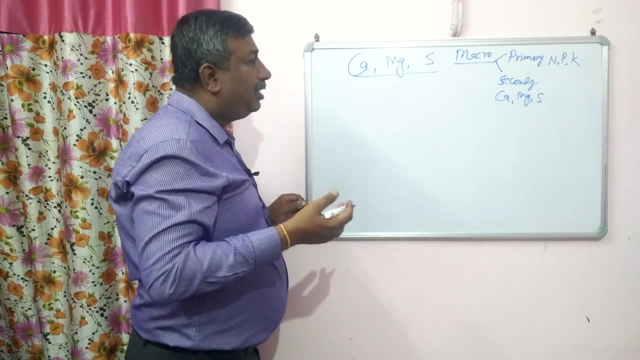 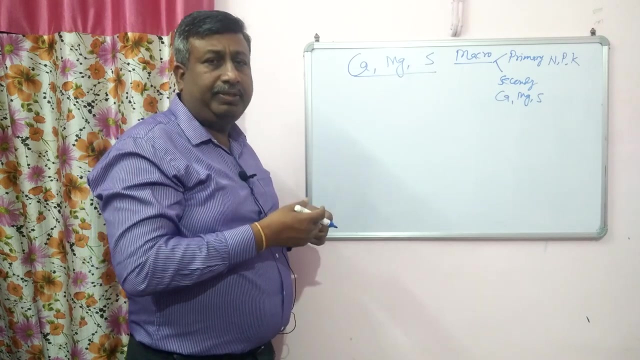 calcium, magnesium and sulphur. because primary importance is on nitrogen, phosphorus and potassium fertilizer, we give primary importance. that's why these are known primary nutrient and calcium, magnesium and sulphur are present in this primary nutrients as a primary nutrient, as a material or as a constituents. that's why importance for application is secondary. so known as secondary nutrient, And plant absorb calcium in the form of calcium divalent form, magnesium in magnesium plus plus divalent form, and sulphur. in case of this sulphate ion, this is the plant available form, so these forms are very important. So 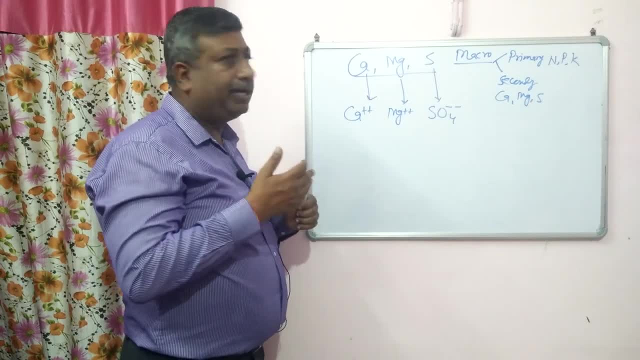 what we are calling calcium, magnesium and sulphur is called secondary nutrient, although this is a requirement of macro nutrient. So this is very important. it has more value. there are two in the macro: primary, secondary and secondary, because when we give fertilizers there are some parts in the primary fertilizers. 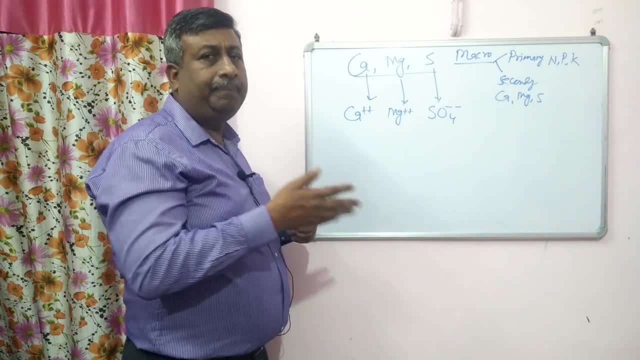 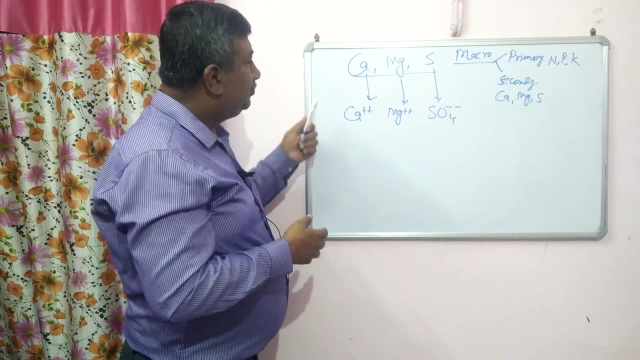 like if we give SSP, then calcium, sulphur remains in it. so secondary importance for their fertilizer application, primary importance for nitrogen, phosphorus and potassium. they are called primary and this is its. this is the plant available form and it remains in. 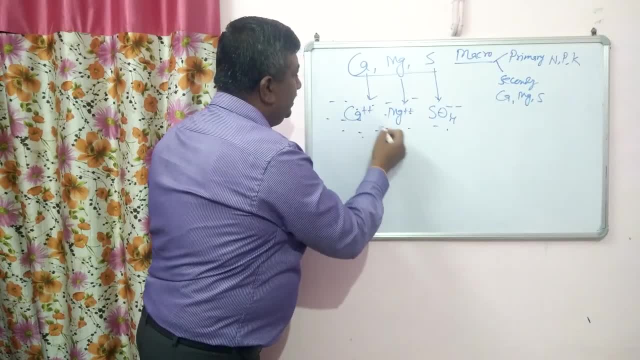 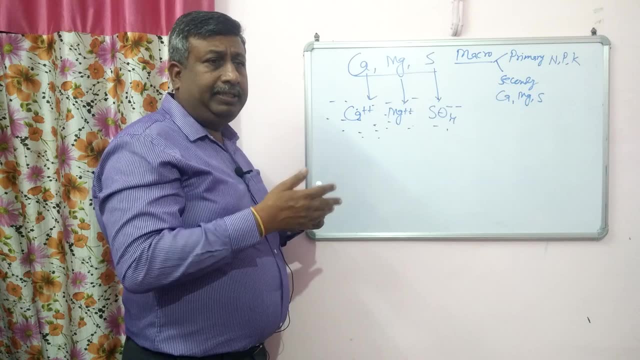 soil solution. if they remain in this form, then these are easily available to the plant. but ions are not in one form, they are hydrolyzed, precipitated. they are not in one form. they are very easily available to the plant and they are adsorbed. so any nutrient does not stay in such form. its form keeps changing. 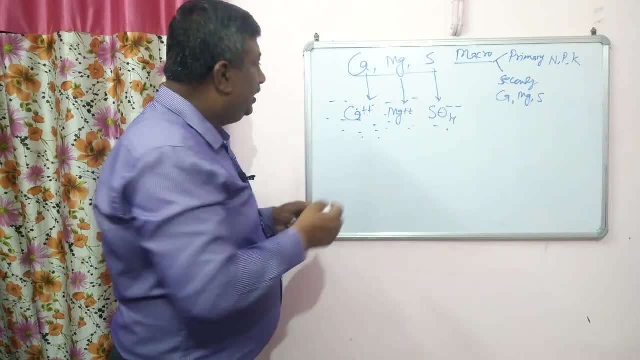 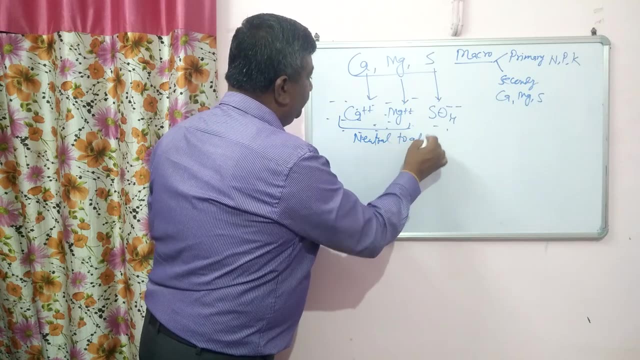 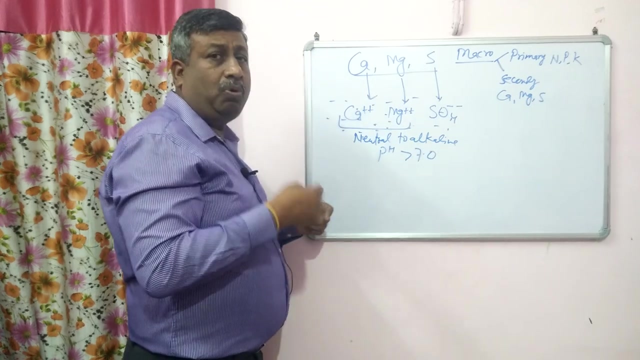 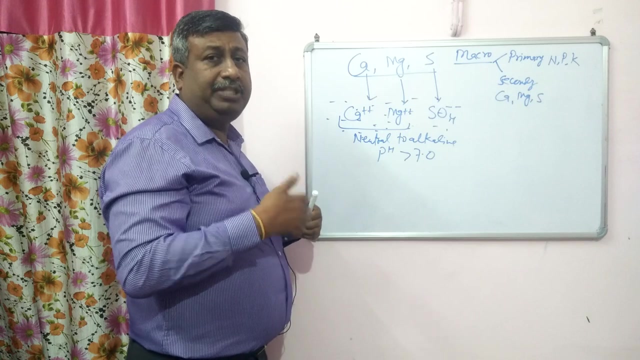 precipitates, adsorbs, leaches, and this calcium and magnesium actually are available at neutral to alkaline condition. When pH is more than 7,, then this calcium and magnesium are more available to plant. Calcium and magnesium both have the same behavior and availability at pH more than 7.. And these are the basic cations. we can say basic cations, calcium and magnesium make the base. they make the base calcium hydroxide, magnesium hydroxide. so these are base forming cations and availability is more than 7 because at pH more than 7, they remain in soil solution in the form of calcium ion and magnesium ion. 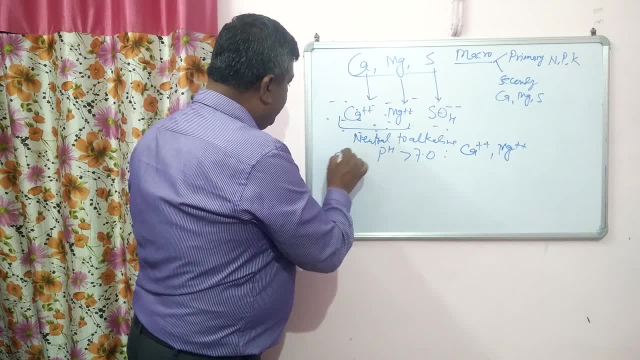 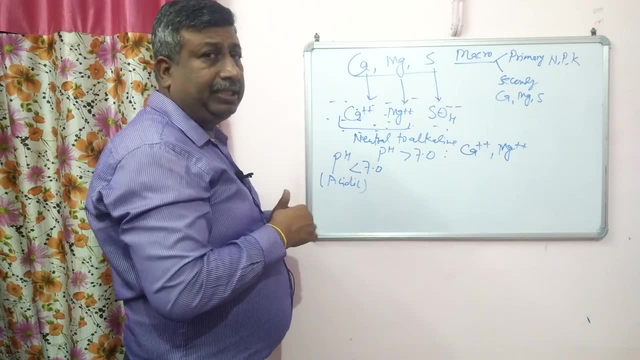 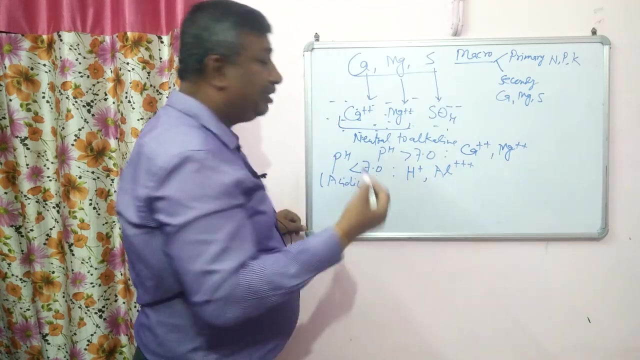 And this is the plant available form. What happens if pH is less than 7?? So under acidic condition, if pH is less than 7, then under acidic condition there is a dominance of hydrogen ion and aluminium ion. So acidic soils produce more hydrogen and aluminium ion, and if soil is organic, then it produces more hydrogen ion. 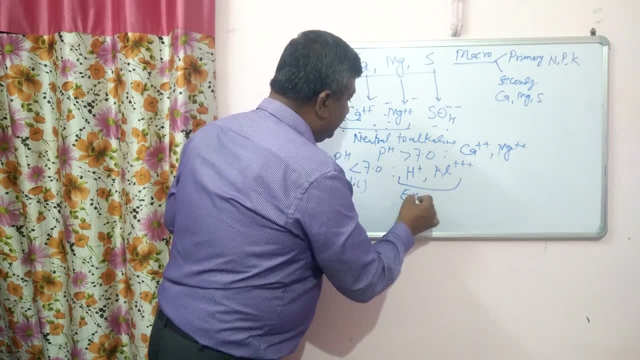 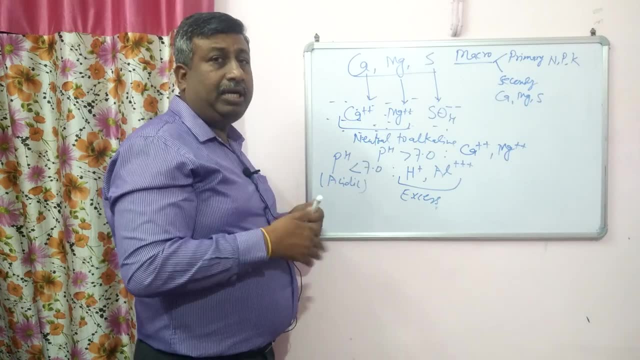 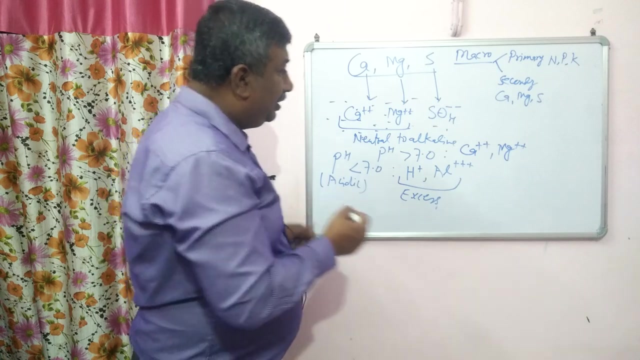 So there is a problem of axis axis, aluminium and hydrogen ion, So they dominate. So in acidic soils there is more hydrogen, Aluminium is present in more soil solution, Iron is also present in soluble form And these dominate. And on the clay complex, actually, so suppose this is the clay particle. 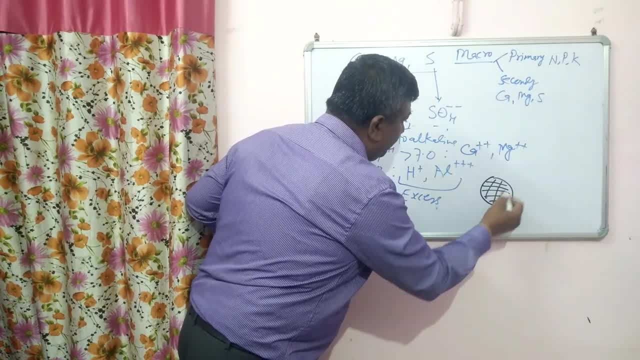 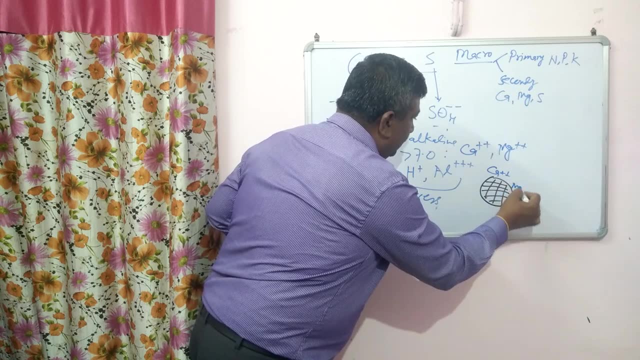 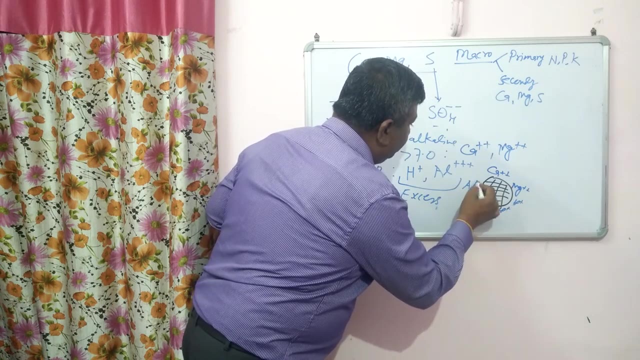 this is the clay particle or humus particle or uranium matter particle, And these carry a negative charge. So suppose there is a calcium and magnesium are present on this complex. Calcium and magnesium are present, Then hydrogen replace Hydrogen, because there is a dominance of aluminum and hydrogen. so that's why they replace. 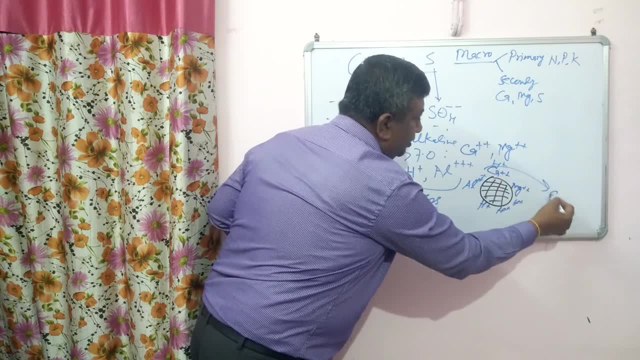 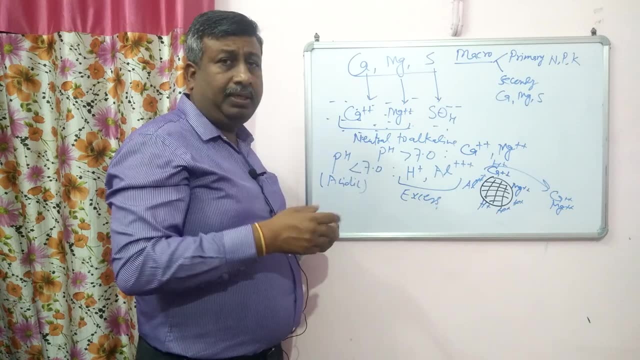 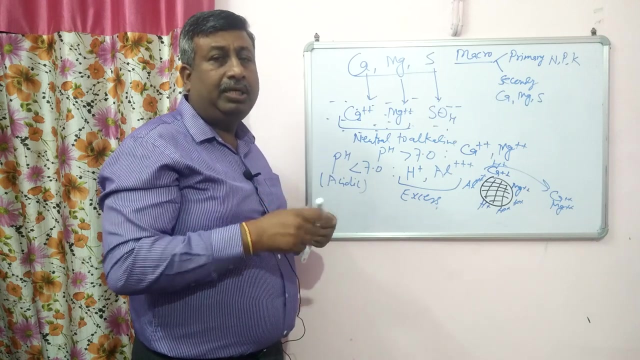 this calcium into the soil solutions. there is a hydrogen, then calcium come into the magnesium. magnesium and calcium both come into the soil solution. so jab yeh itne jyada availability ho jatiye acidic condition me to acidity, hotiye hydrogen ions hai to acidic condition iska madla wahan hydrogen ion hai. 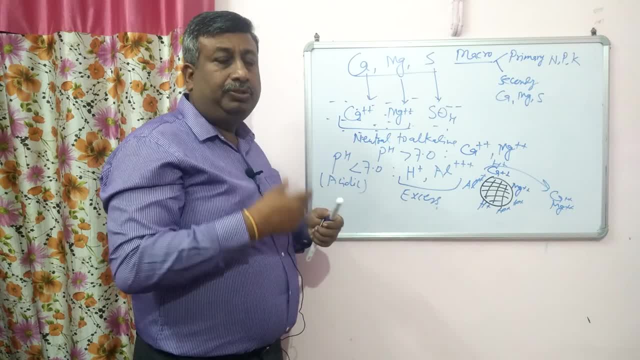 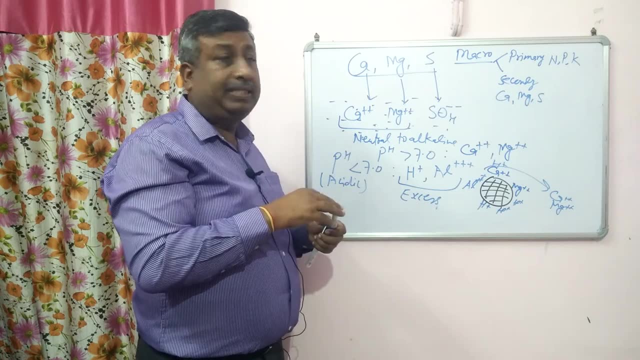 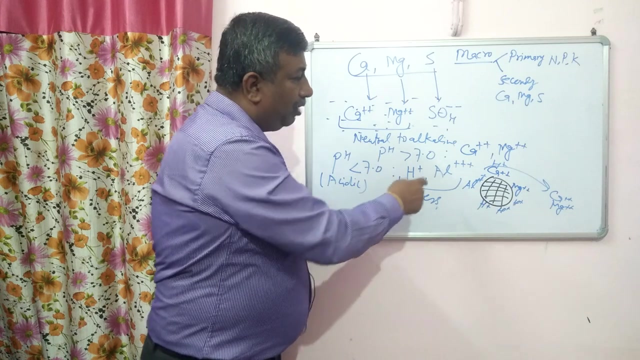 aur acidic condition me aluminum jyada soluble ho jyata hai jo iski precipitated form hotiye high pH, pe wo acidic condition me soluble ho jyata hai to aluminum becomes more soluble under acidic condition and when these are soluble and in ion form. aluminum is now present as tribal and form, so ab kya. 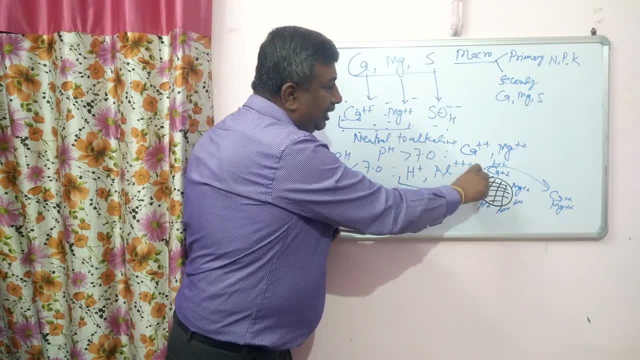 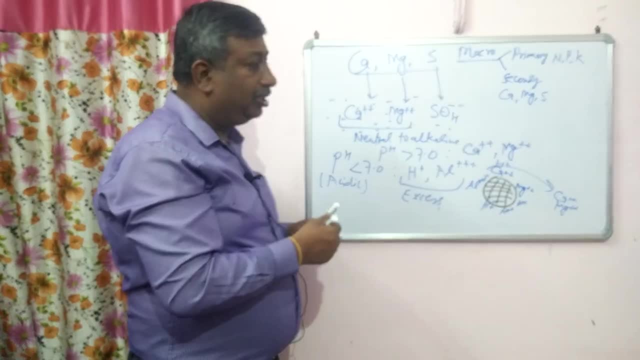 karenge. they come on to the exchange complex, jo clay particle, humus ka hai. they come on to the clay complex and they replace the calcium and magnesium, and this calcium and magnesium come into the soil solution and there, with the percolating water, they leach down. so leaching is there, so 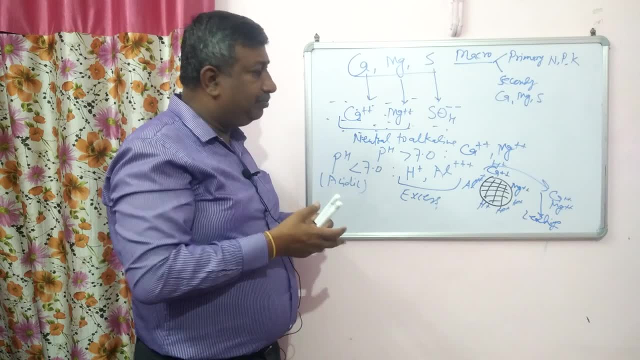 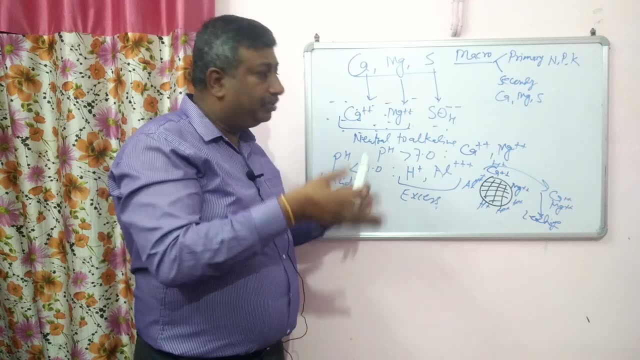 they are not adsorbed. there are no mechanism to adsorb because there is a dominance of hydrogen ion. ab itna jyada hydrogen or ammonium hai ki isko replace kar deta hai exchange complex to the soil solution. mein aate ab inko kahin jaga. 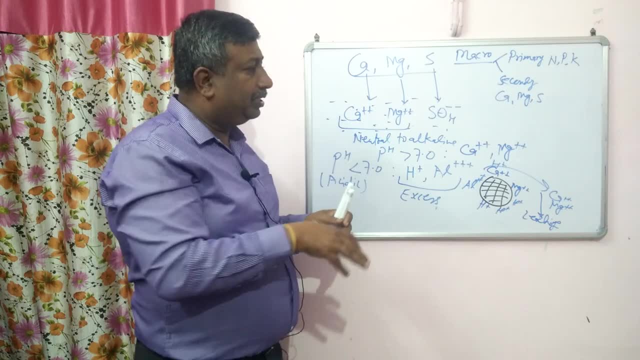 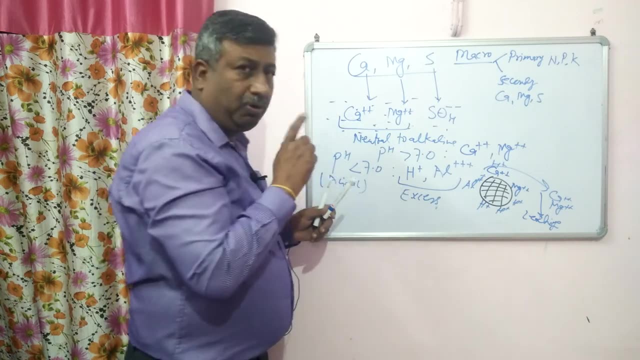 nahi milti calcium and magnesium ko to paani mein aate hai. aur jase hi water percolate karta hai. they percolate with the water- that process known as leaching. so there is a competition. so low availability of calcium and magnesium in acidic. 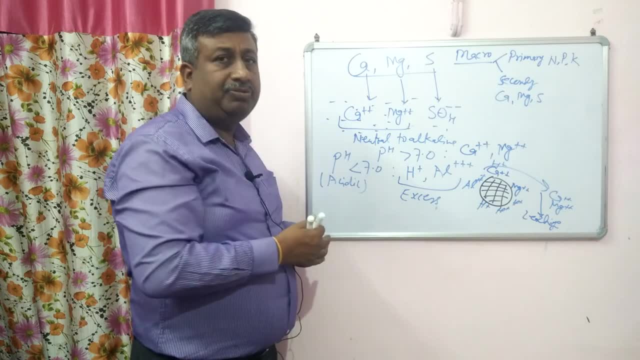 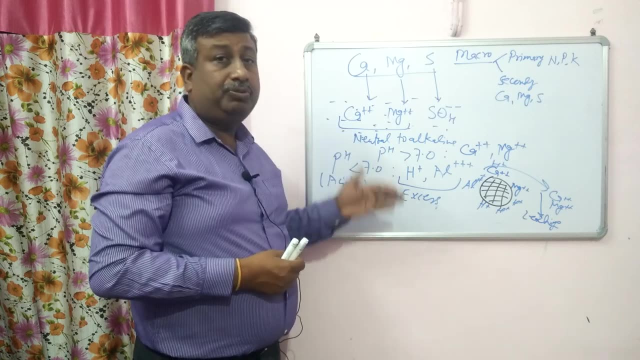 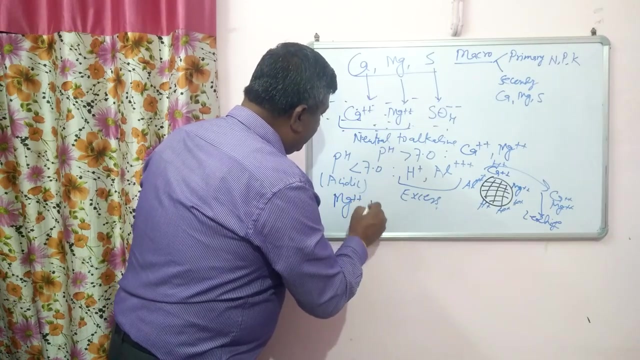 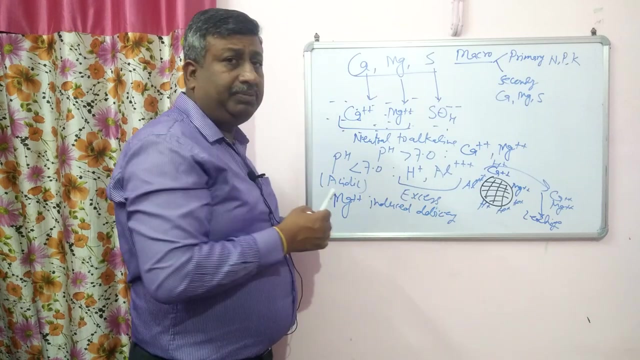 condition is because they face the competition from the hydrogen and ammonium ion. so this is the reason that there is a deficiency of calcium and magnesium ion. or we can say acidic soil produce induced deficiency, particularly magnesium. so this is a magnesium induced deficiency, magnesium induced deficiency. so acidic soil produce the magnesium deficiency down. magnesium is present to. 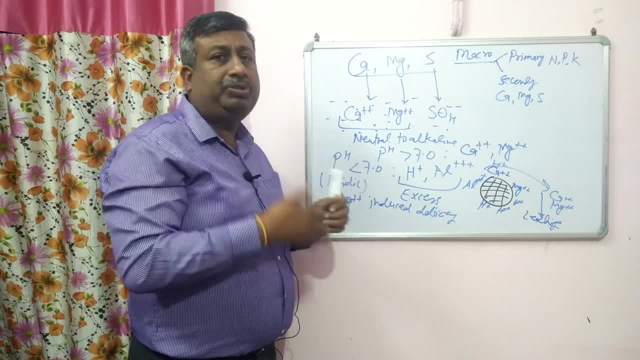 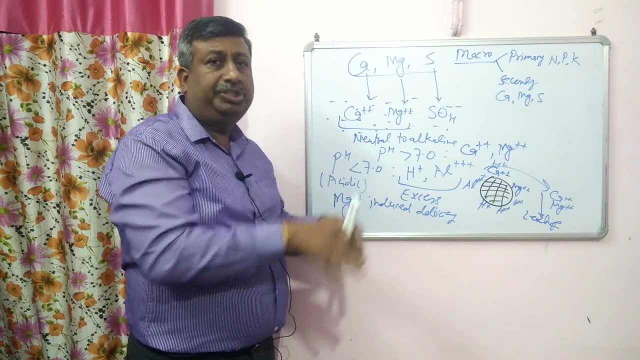 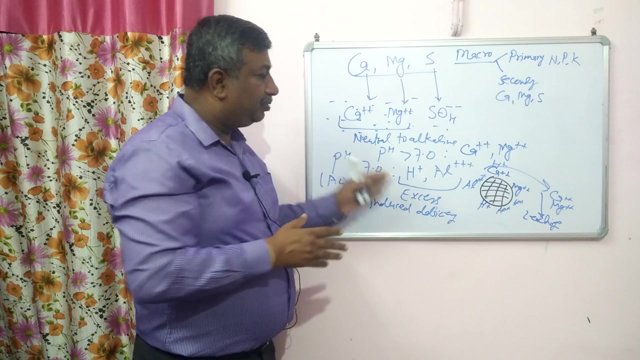 you a common is acidic soil. it induces deficiency, however. it is present in soil but it is happening, So it is very common. magnesium induced deficiency in acidic soil is very common. So the reason is dominance of hydrogen and aluminum ion, which replace the calcium and 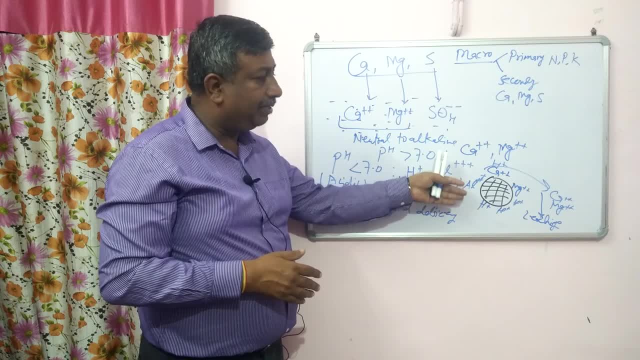 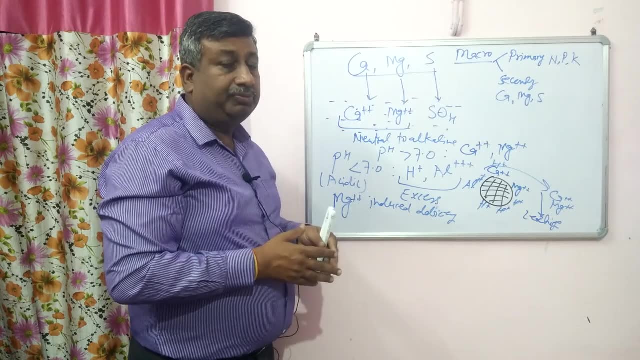 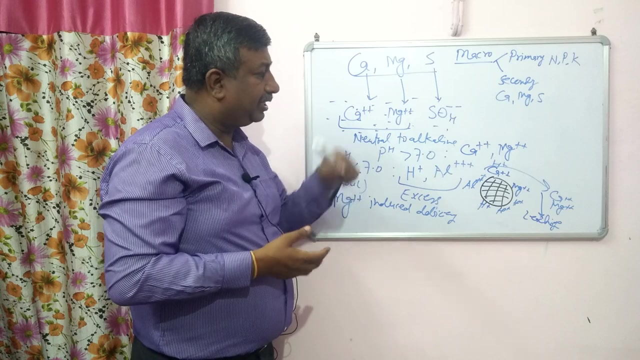 magnesium from the exchange complex means clay collide, humus collide or organic matter and they come into the soil solution. daily is down. that is why there is deficiency of calcium and magnesium. So actually this is the induced deficiency, But at pH more than 7 they remain in soil solution in this cationic form and available. 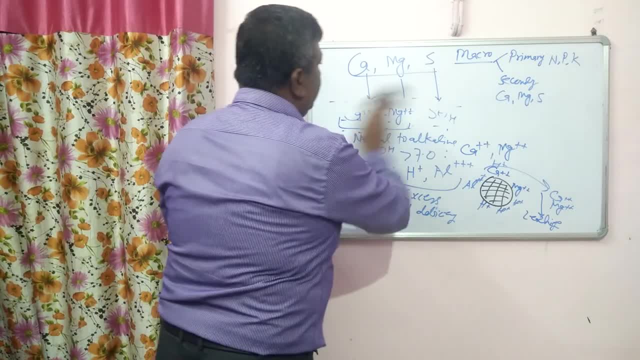 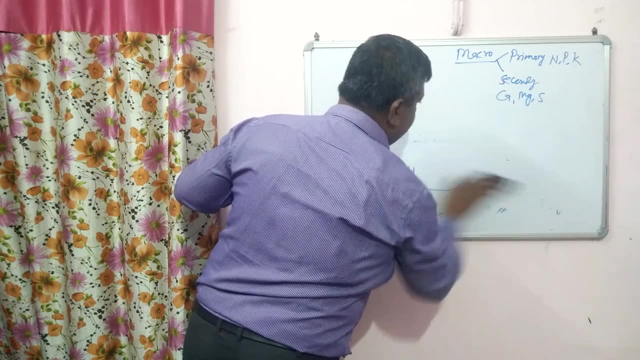 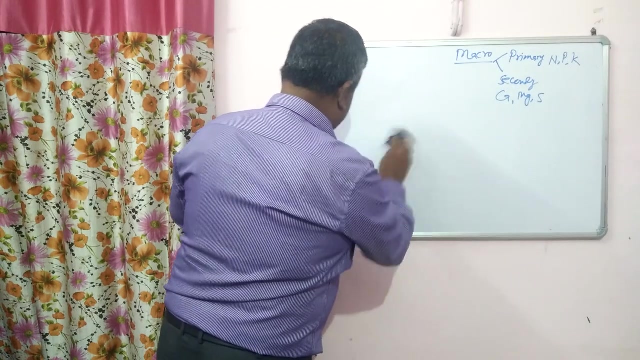 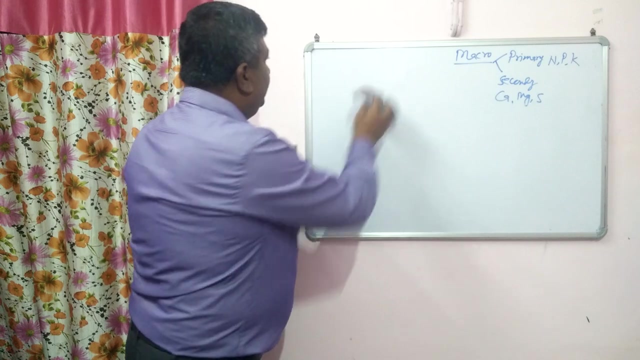 to the plant. So this is the reason that calcium and magnesium are more available at high pH and under acidic pH. their deficiency is common. Now, in case of sulfur, sulfur is available in the form of sulfate ion, SOO4. And this sulfate all anion and this is the available form sulfate. 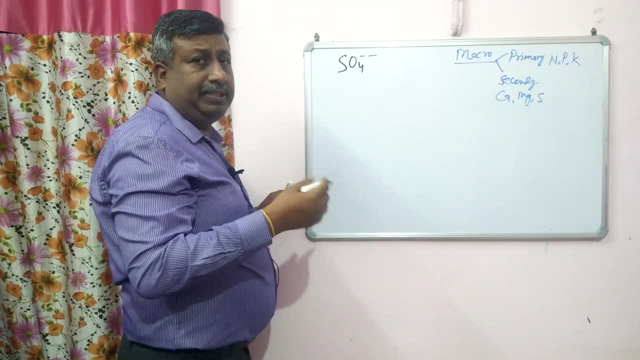 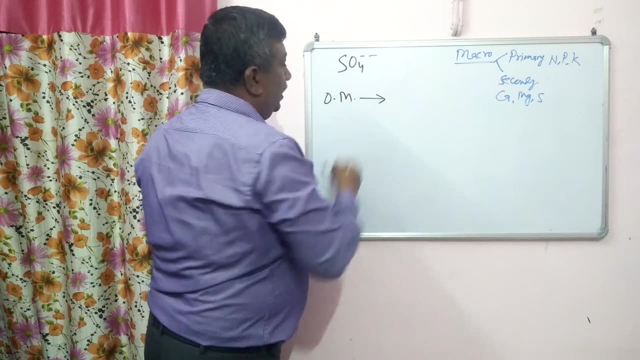 The available form of sulfur is sulfate ion and sulfur is present in many forms in soil solution, And this is actually organic matter- is the source of sulfur, Actually, in plants sulfur is present in amino acid like Cysteine, Cysteine and methane. 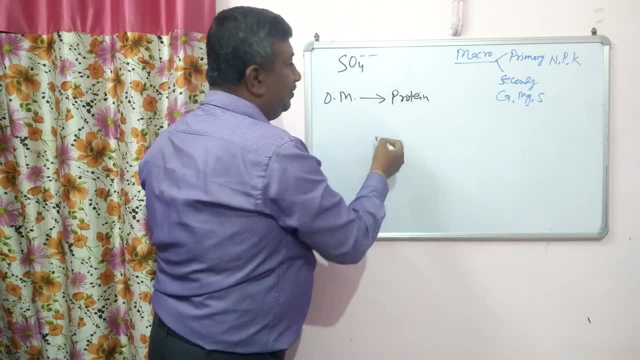 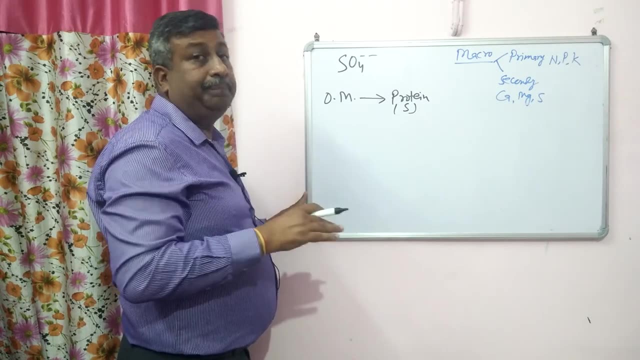 So it is present in organic matter as a protein, Because there a sulfur containing protein protein. So nitrogen and sulfur, both are required for protein formation. So sulfur bhi chahi hota hai, kyunki, cysteine, cysteine, methionine, amino acid mein form hota hai. Then 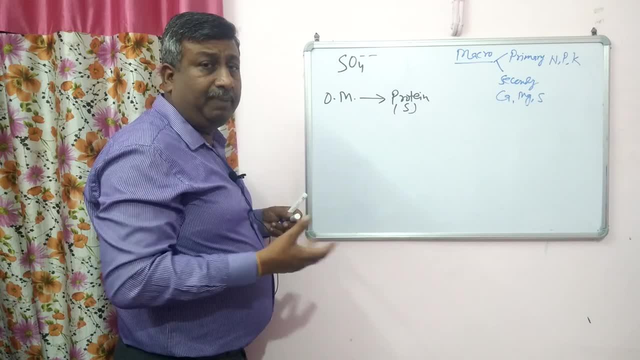 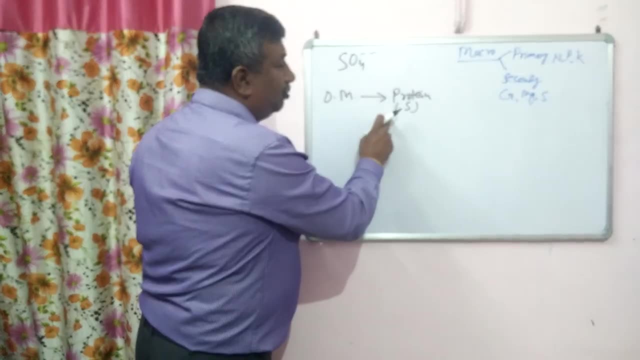 it is also present as a sulfonic acid. It is present as a sulfolipids: Lipids mein rata hai, Sulfur usmein rata hai. There are different form of sulfur in organic matter. So organic matter is a good source of sulfur. So this sulfur ability depends upon the organic matter. content. If soil has more organic matter content, it means sulfur availability is more. Even 75-80% sulfur is present in organic matter. Even more than 80% May be more than 80%. So it means our nitrogen case same hi rata hai Nitrogen remain 95-99% in case of nitrogen. 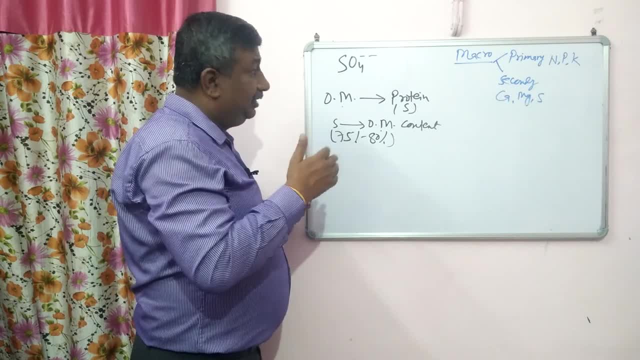 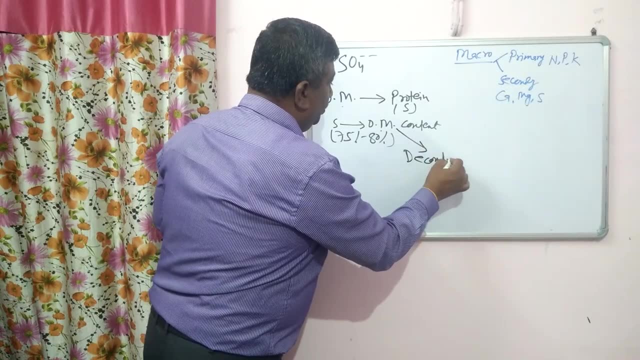 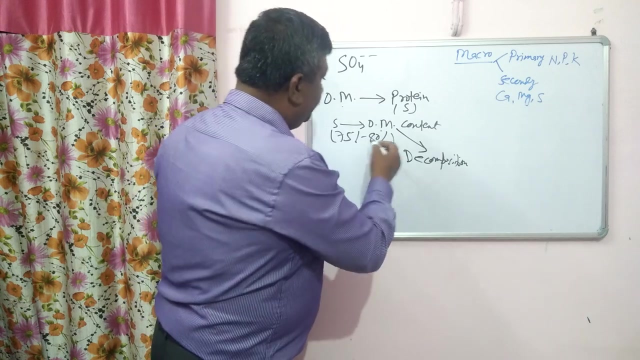 So behavior of nitrogen and sulfur is same, If we see the availability. So there is organic matter decomposition. There is organic matter decomposition, Then there is a- I am not sure what it is, I mean acids right on to peptide and then release of sulfate ion, So decomposition. 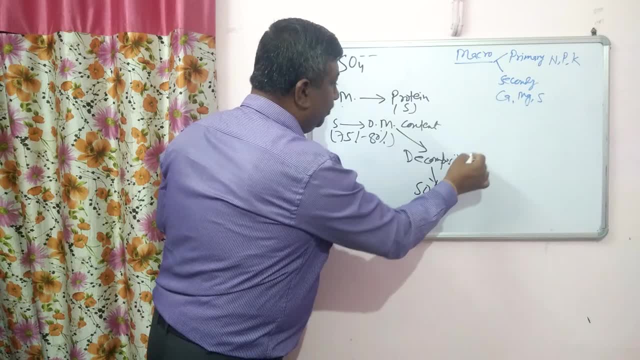 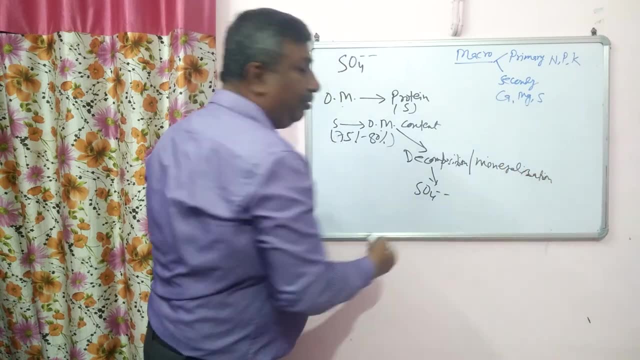 is there and then sulfate ion relays by the decomposition and the mineralization process. we can say Mineralization. So if there is a mineralization then there is a more availability of organic matter because there is high content of sulfur in organic matter. 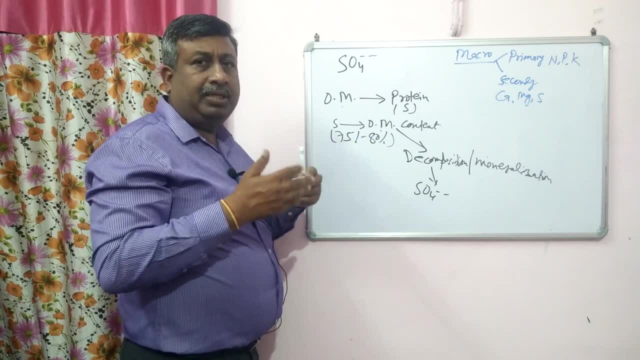 Aba organic matter ke andar sulfur hota hai, Leaves ke andar stem ke andar Inmei sulfur hai, kyunki sulfolipids hai Membrane mein hai Sulfolipids hai kahi sare compounds hota hai. 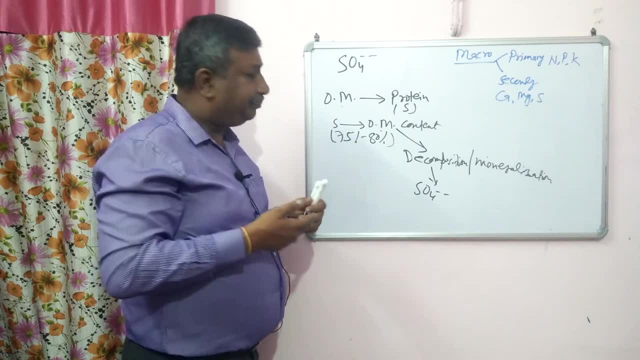 Aur jo particuli게, salicylic acid, as well as spirits which are present in organic matter, So particularly proteins which contain amino acids. so this means that the organometer is a very good source of sulphur, and sulphur is generally obtained from the organometer. Now, when will this release? Sulfur, just like nitrogen, when it will decompose. so the behaviour of nitrogen and sulphur is the same. Now, if there is decomposition, then sulphate ions will be released, and this decomposition is mediated by microbes, bacteria. many bacteria are involved in decomposition and mineralisation. 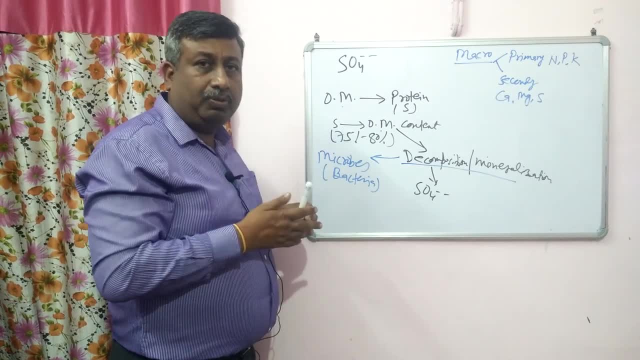 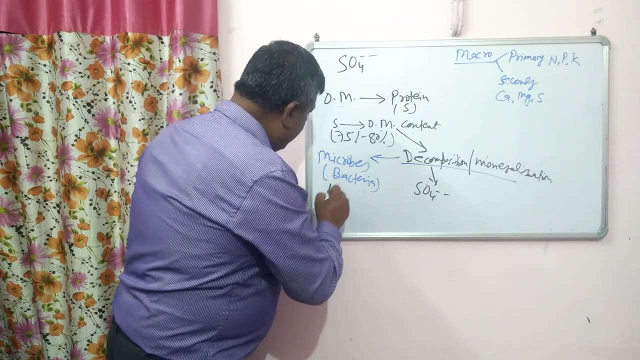 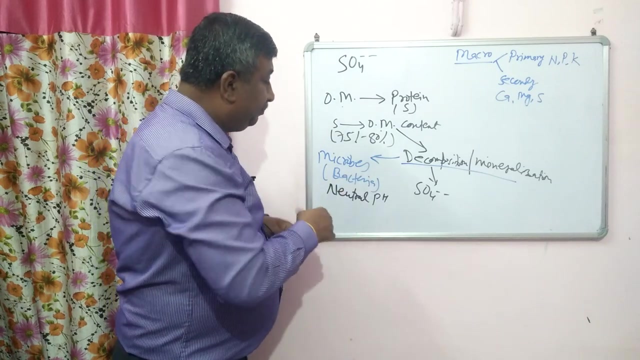 of this sulphur. So now this organometer will decompose, bacteria will decompose and then these sulphate ions will be released And bacteria work at a neutral to alkaline condition. we can say neutral, So at a neutral pH there is a maximum activity of bacteria. that's why more availability. 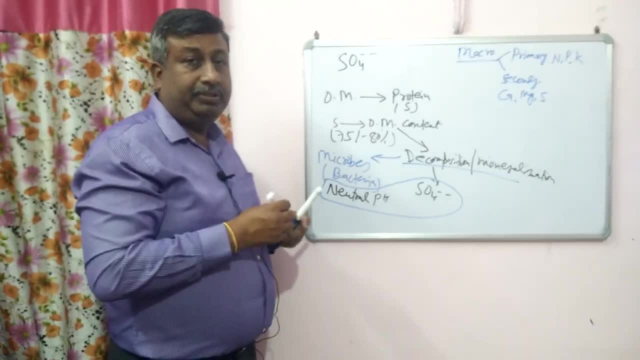 of sulphate ions And sulphur is at a neutral pH. So this is the reason that maximum availability of sulphur is at a neutral pH, as like in case of nitrogen. Like in case of nitrogen also, there will be maximum availability of sulphate ions at a 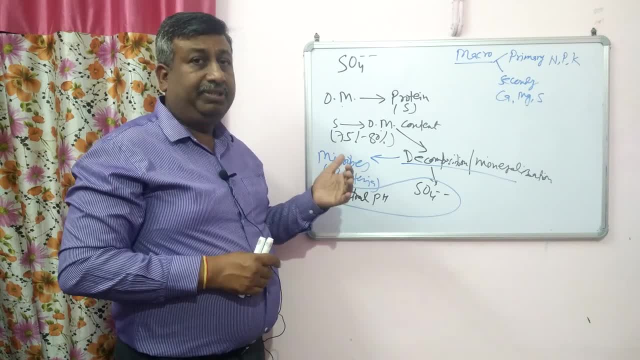 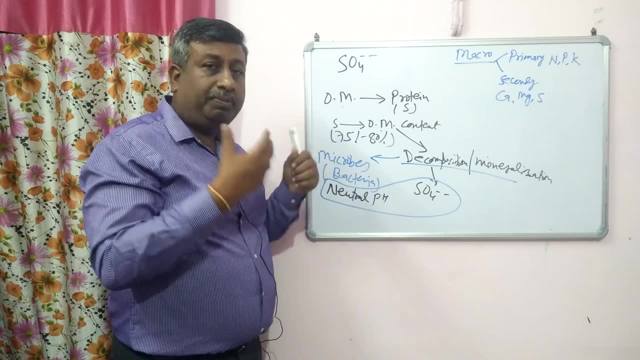 neutral pH Because of the activity of nitrosomonas nitrovector. there will be more mineralisation Here. there is thiobacillus. there is a very important bacteria, thiobacillus. its activity will be there, decomposition will be there, mineralisation will be there. there are other. bacteria which are involved in decomposition of organometer and release the sulphate ion or sulphur mineralisation. we can say So there is a maximum activity of microbes at neutral pH. That's why sulphate or sulphur availability is at neutral pH Under acidic condition. at alkaline condition, sulphur availability is reduced.